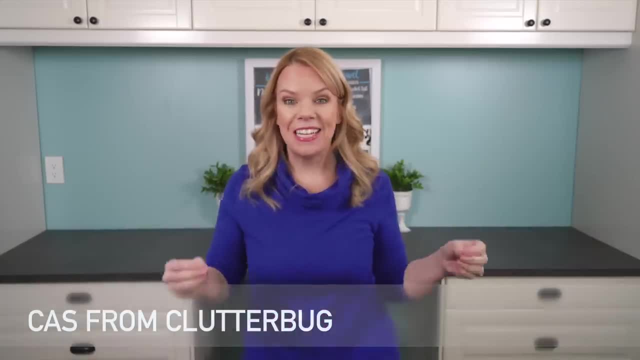 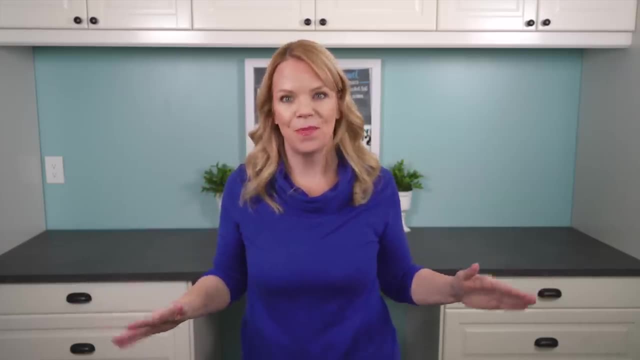 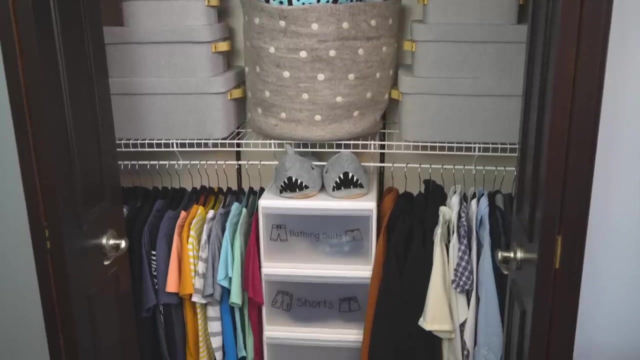 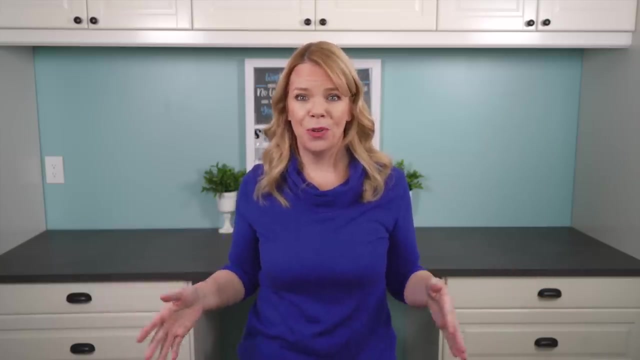 Hi and welcome back if you're new here. I'm Cass from Clutterbug, and today we're talking about the five real life steps that you need to take to get a totally organized home. No matter what area of your life you want to improve, an organized home can help because 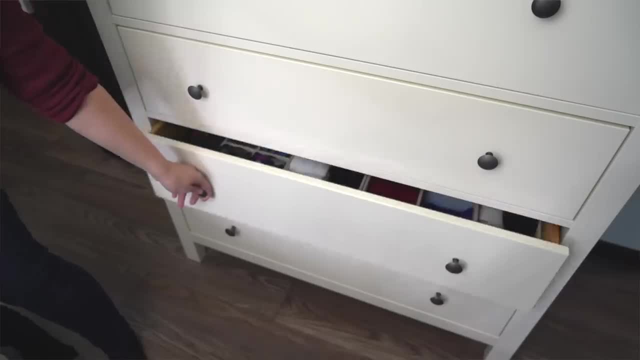 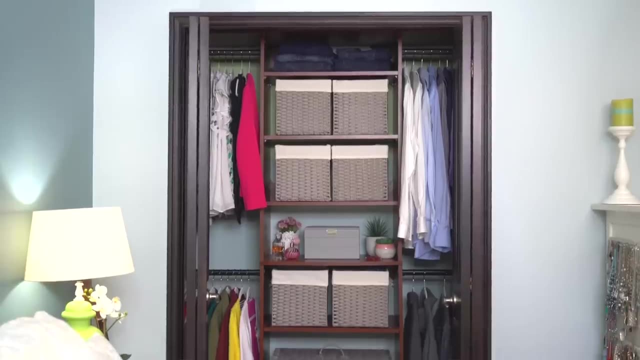 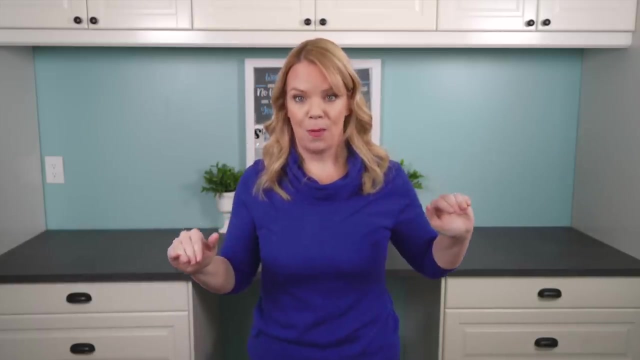 your home is like the foundation for your entire life, And when you're in control and it's solid, everything improves: Your relationships, your finances, every aspect, your self-confidence more than anything else. And I know this because I used to be a super slob And when I finally made 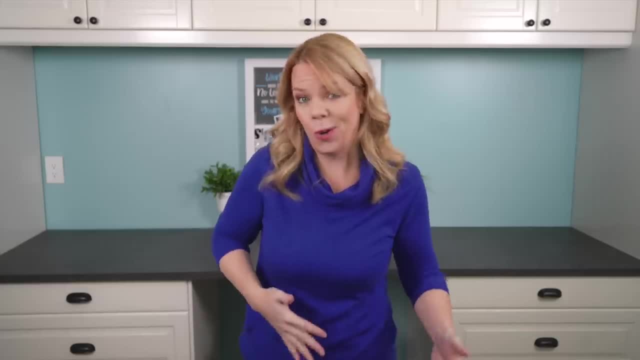 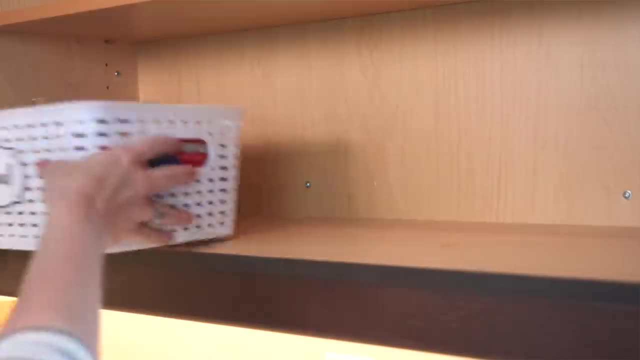 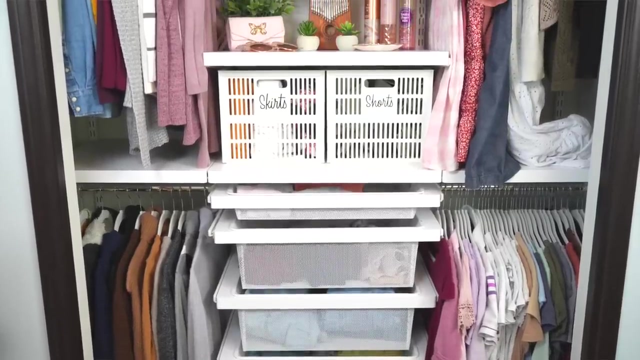 that transition to organization. it's badonkadonks crazy how much my life improved, And I want to help you too. But here's the thing: It isn't just going to the store and buying containers. We can't just solve the problem by spending more money and buying more stuff. There's actual, real. 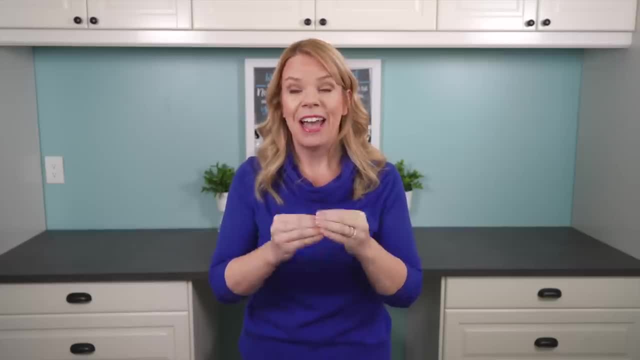 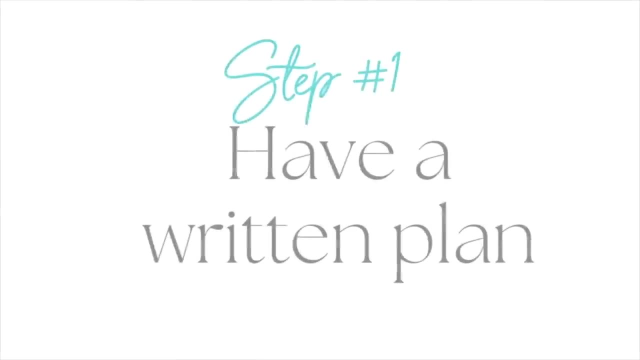 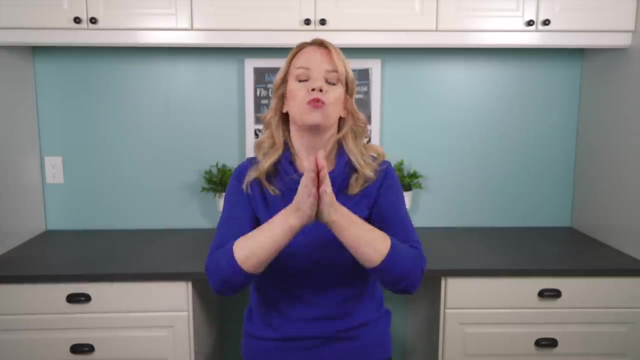 steps to transforming your home through organization, And I'm going to share those with you right now, starting with the very first one, And this one is critical. The first step is having a written plan. A goal without a plan is just like a dream. We have to actually write down. 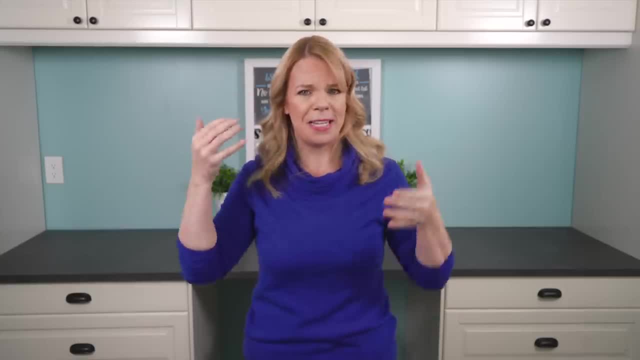 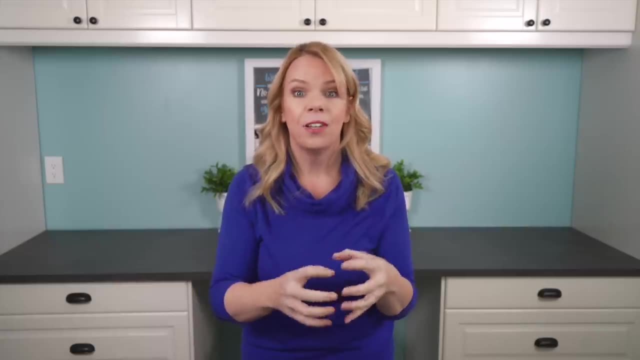 the thing that we want to accomplish. Not only does this shift things in your mind and make it a goal, but by breaking down that goal into lots of little chunks, you're also way less likely to feel overwhelmed and procrastinate. I call this brain dumping. So think about organizing your. 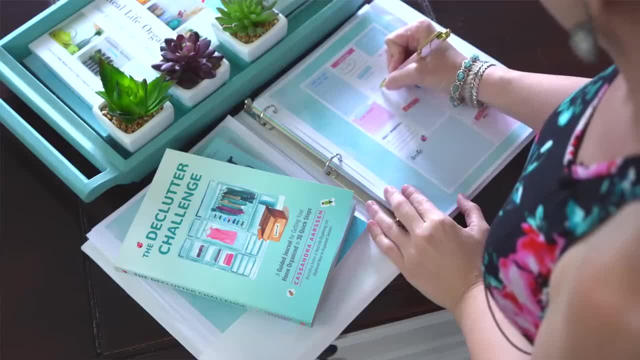 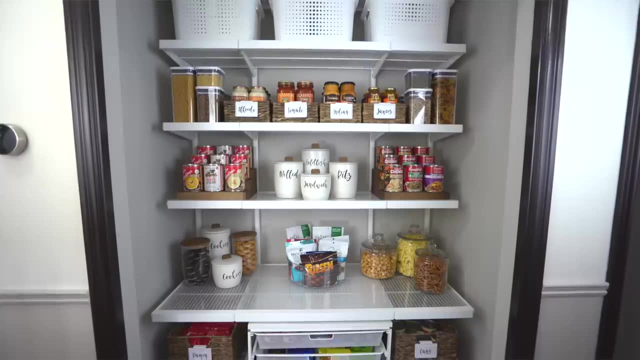 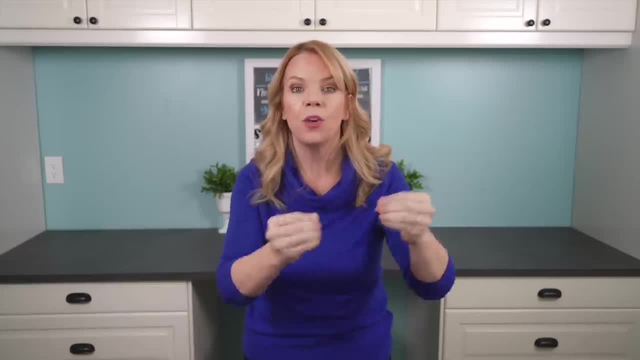 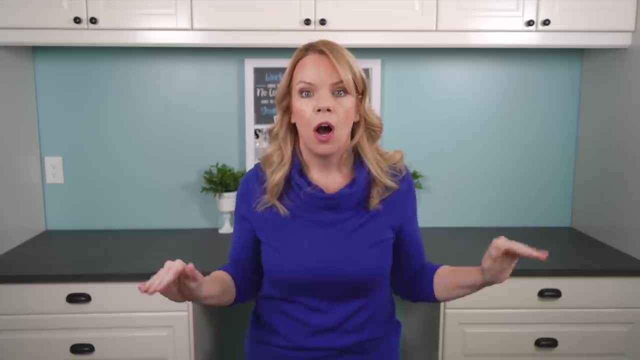 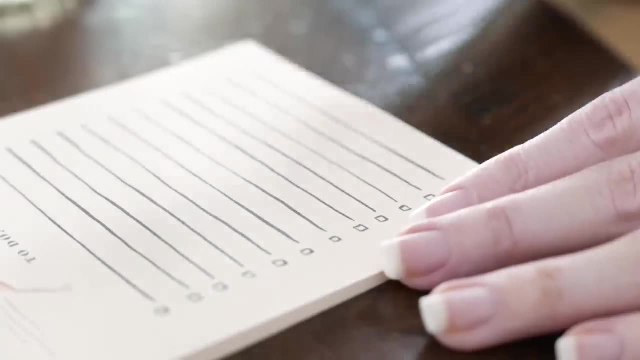 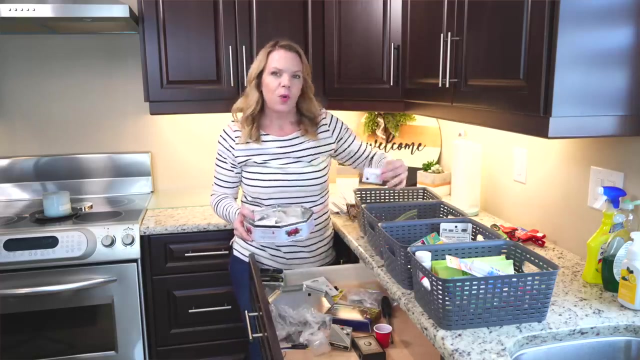 you more than 30 minutes to an hour tops. So one shelf in a closet or maybe just all of your t-shirts. Doing it this way, making a plan, writing everything down, is key to overcoming that procrastination. It's key to shifting your mindset and really declaring what your goal is. 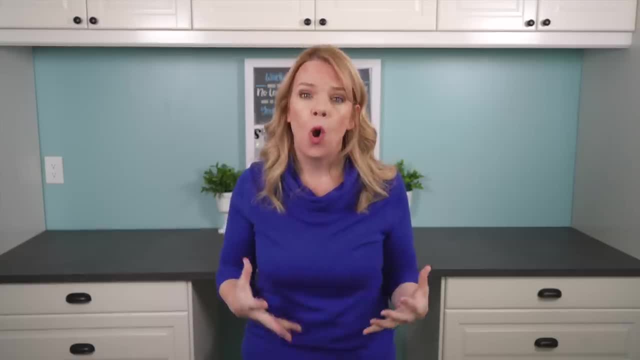 so that you can make it happen. Step two is so critical. This is something that we just don't do. I don't know. This isn't time. It's like time management. Why aren't they teaching us? This is the critical step for seeing success, And that is taking a look. 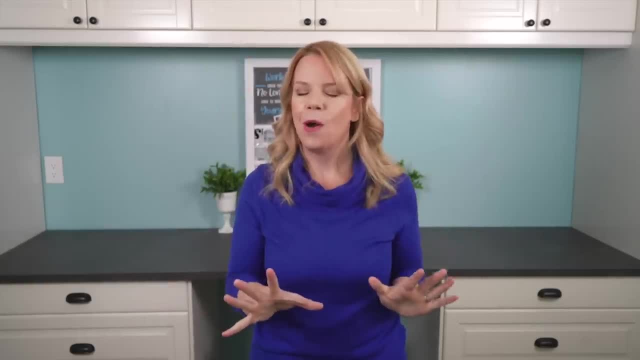 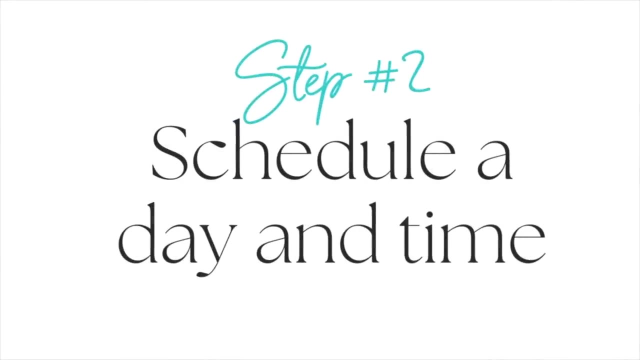 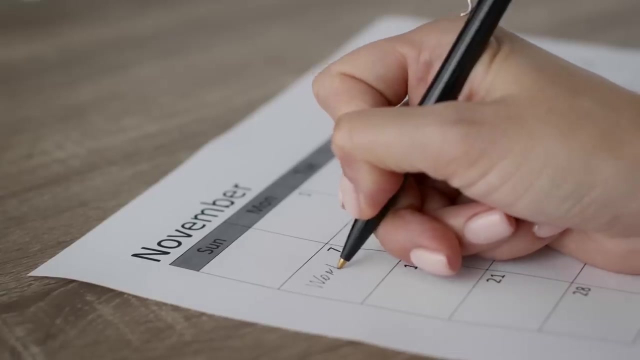 at your big list, all your brain dumps all the things you want to accomplish, picking one and scheduling a date to do it Like picking I'm doing this Friday at 4 PM and put it in your calendar. You can put it in your electronic calendar, You can put it in your planner, whatever you use to. 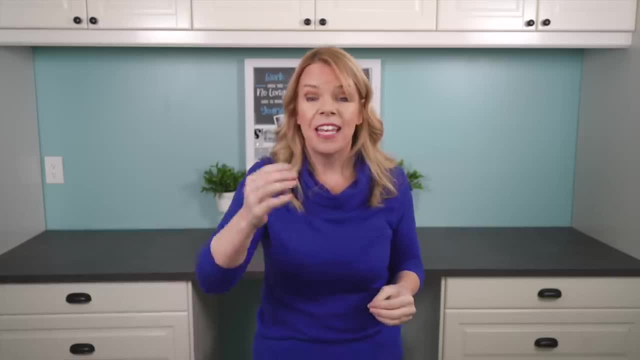 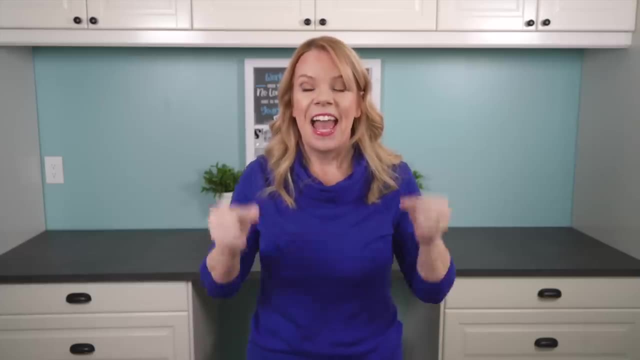 plan your time. You have to schedule a date with yourself because, if not, we're just going to continue to procrastinate this. We're going to put it off and not make it a priority. This is key. Every single thing you want to do, you have to set a date with yourself. I didn't come up with this. 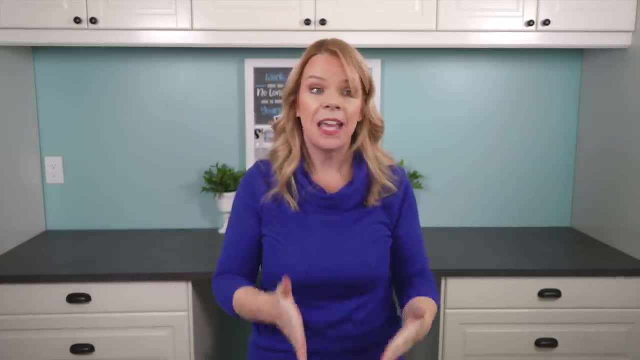 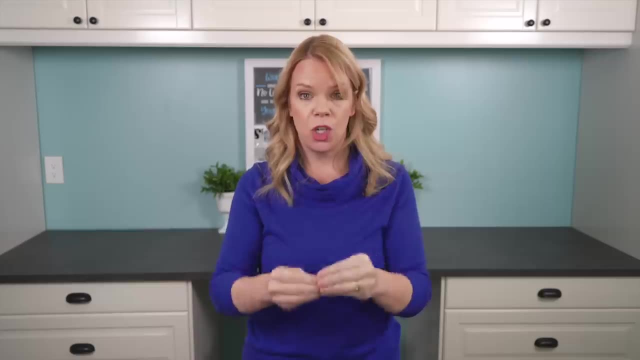 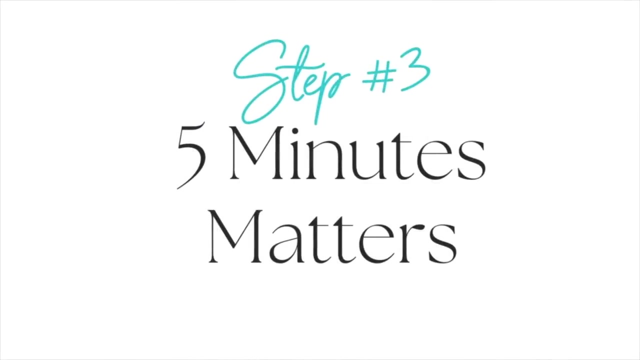 Brilliant time management experts have shown time and time again. research and studies have shown that when you put something in your calendar, when you set a date to achieve a goal, you are way more likely to actually do it. Step three is the mantra: five minutes matters. I'm great about making 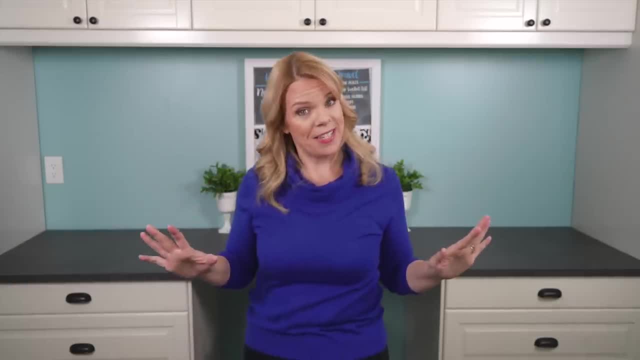 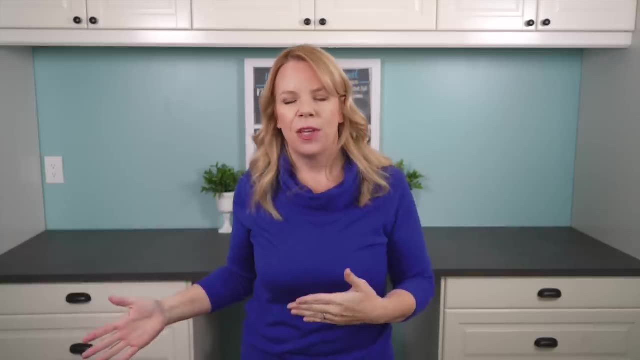 lists. I can make lists all day, but I also tend to procrastinate or like snooze the events. right, I mean, that's human nature. We, we always are looking for the shortcut, the way out of doing the work. but the five minutes matters. mantra means that you just repeat to yourself. I only 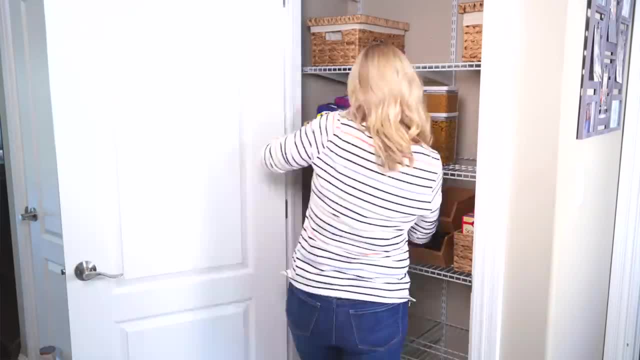 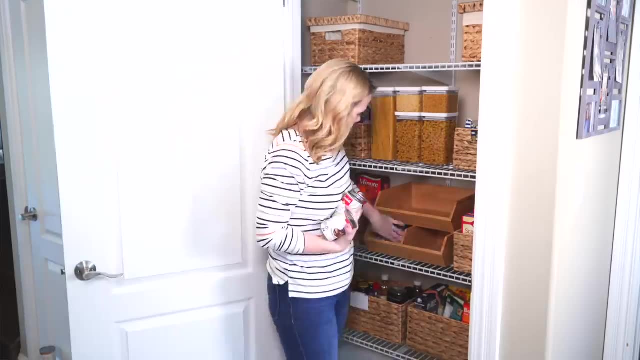 have to do this task for five minutes. Maybe you're supposed to be doing the junk drawer today. You only have to get up and work on it for five minutes. That's it. Set a timer. We can do anything for five minutes, And what this really does is 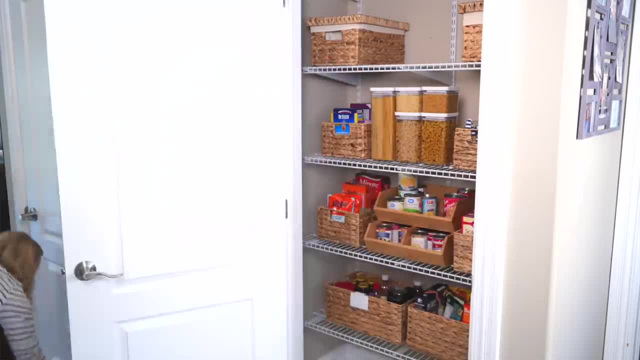 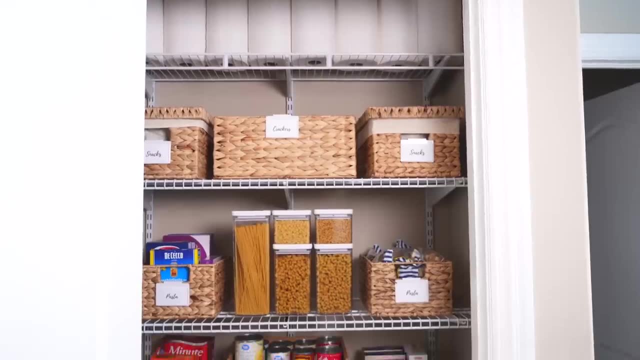 it tricks our brain to get up and get started, And even if we stop at five minutes, we're going to be way further ahead than if we had done nothing at all. But what usually happens is the hard part is getting up. It's getting yourself motivated. But once you have that, 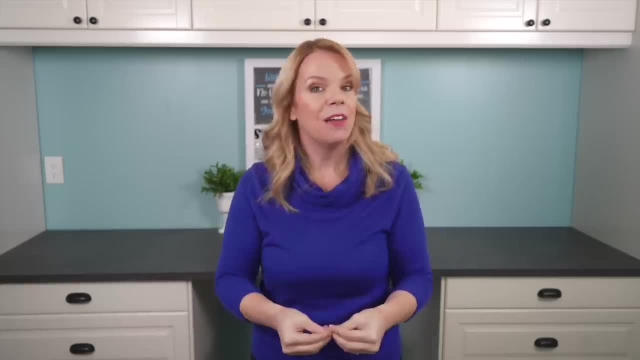 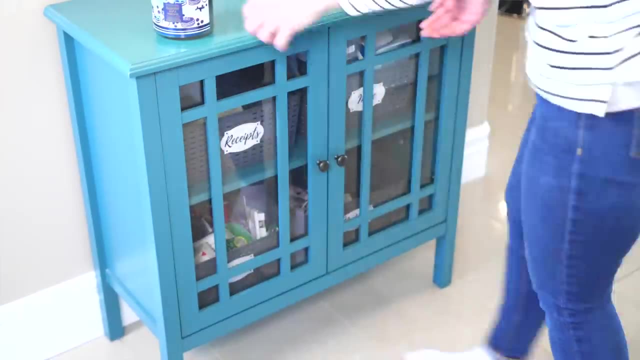 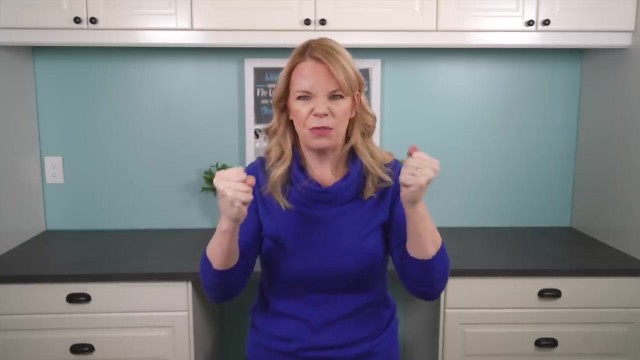 the momentum will carry you through, And so five minutes matters. mantras has changed my life. I schedule things, I write down all the things I want to do. I schedule a date with myself, And when that alarm reminds me that it's time, I grudgingly get up and say: I only have to do it for five. 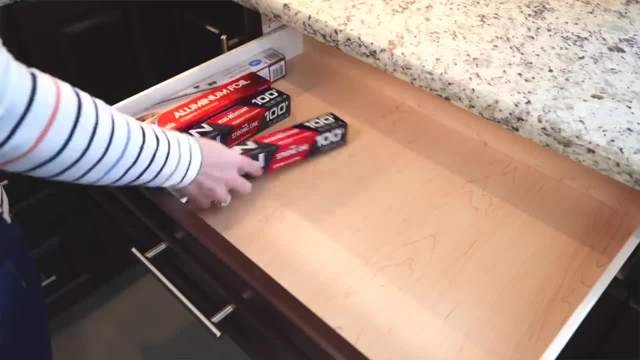 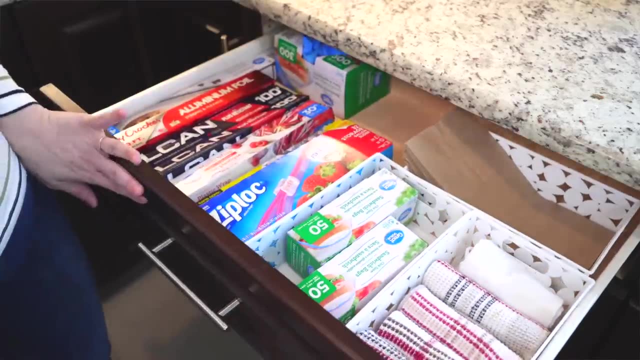 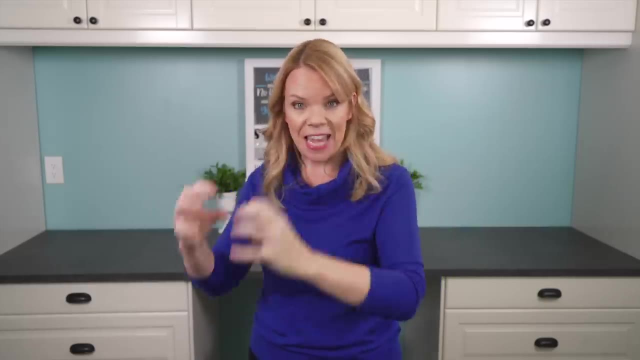 minutes, And the magical thing is, I accomplish amazing things And I've talked to so many incredibly successful people that I respect, And this is their secret: They write down their goals in actionable, small, bite-sized pieces. They schedule a date to do each of those things. 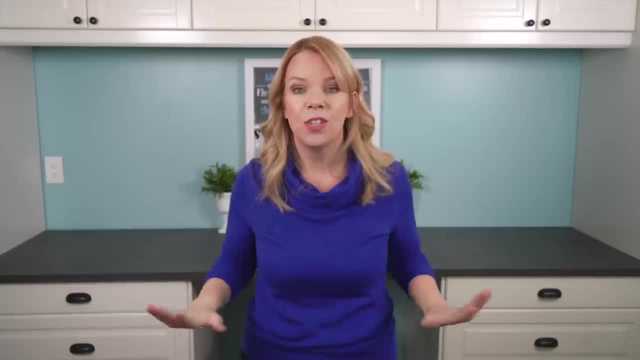 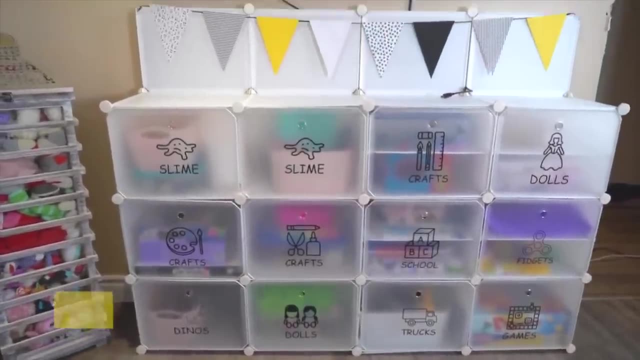 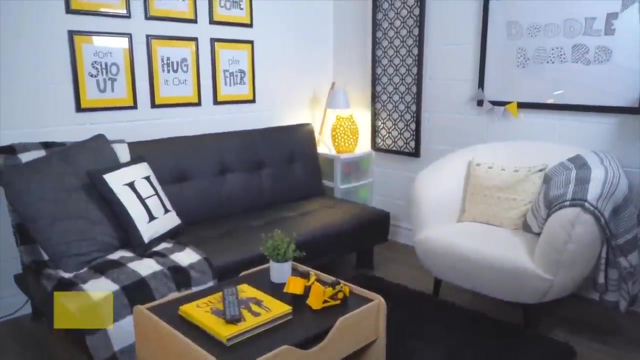 And they force themselves to get up and do it just for a few minutes. Eat that frog. It's called: get up, do it. It isn't about adding a lot more work to your plate. It's about creating a real time management system so that you can have long-term success and that you're in the mindset. 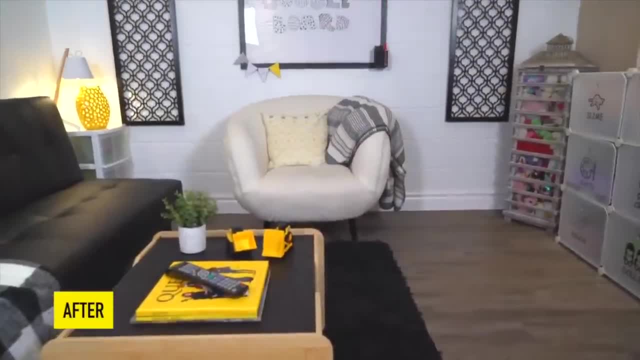 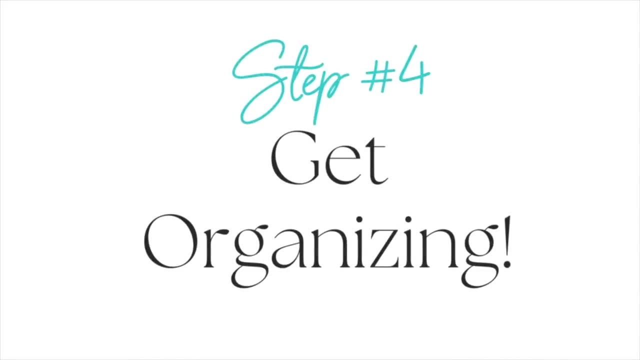 of like it's go time. I'm going to take back my house. I'm going to organize the space because I deserve it. Step four is the actual organizing part. You can try to jump right to this, but this is why we fail. We have to do the planning, That's. 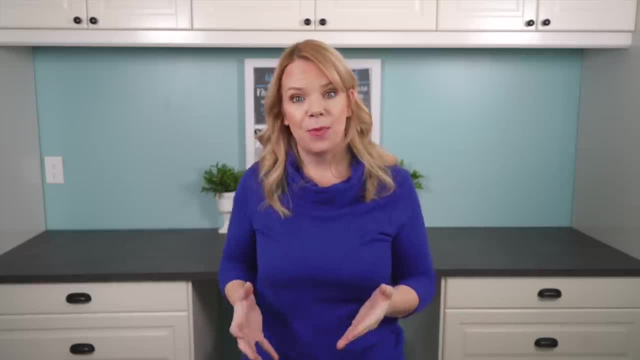 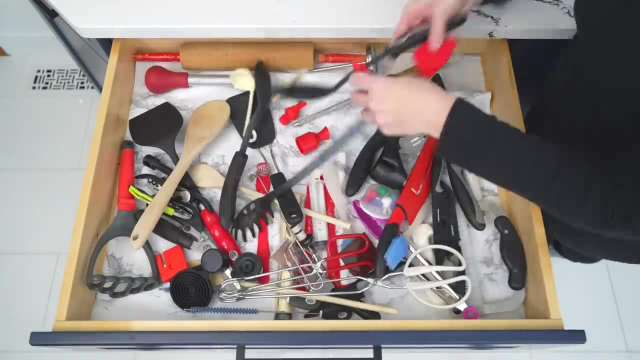 like 90% of the job is the planning. The organizing part is actually the easiest part of this, but here's how we organize properly. We start with whatever space, whatever small task, and we take everything out, everything out of the drawer, everything off the shelf. 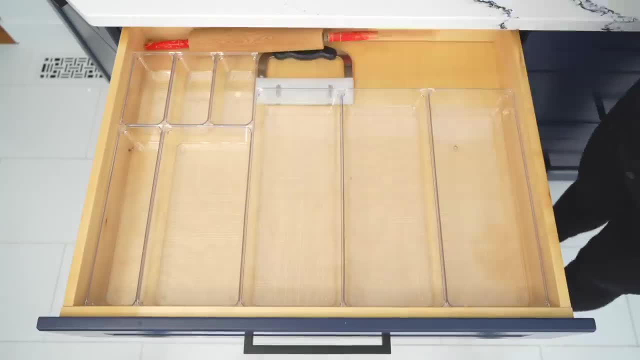 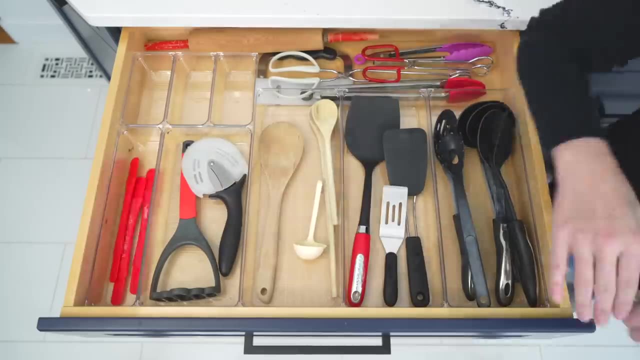 not your whole kitchen, not your entire closet. one small project at a time. Take it out and now put things back, starting with the things you use the most often. We always start with the things we use the most often because that's fun. It's like shopping our 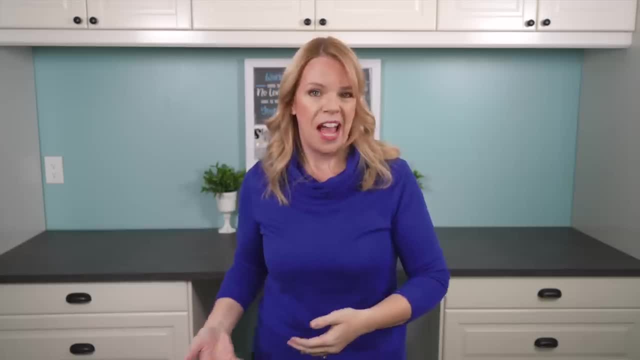 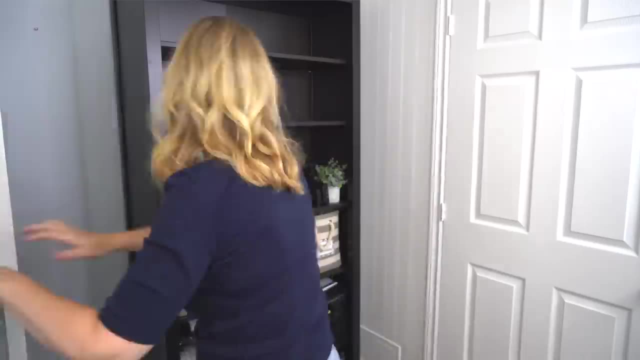 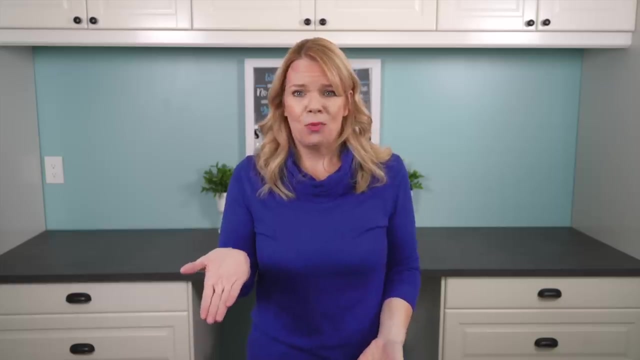 stuff, but it also really shows us what we don't need, And you're going to find a ton of stuff that can go. This is so important: to declutter. We can't organize excess, So as you're putting things back when there's random things left over, you're like I don't know where this should go. Why is it? 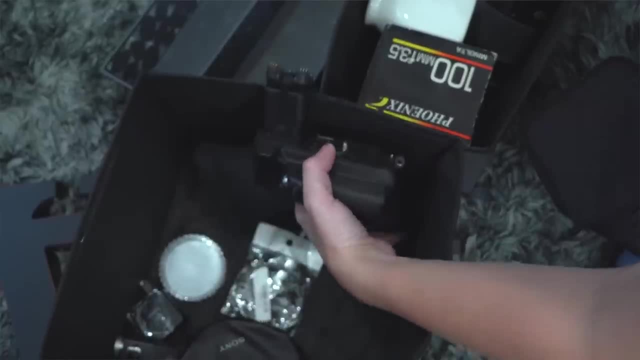 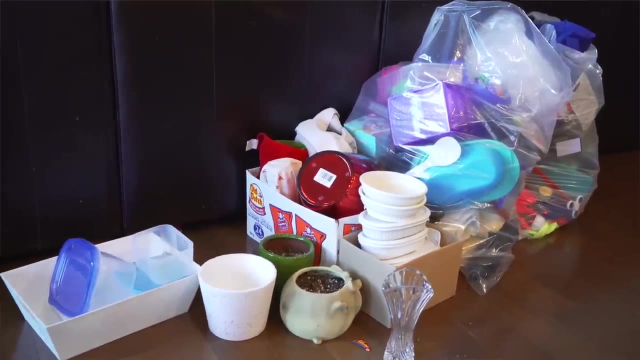 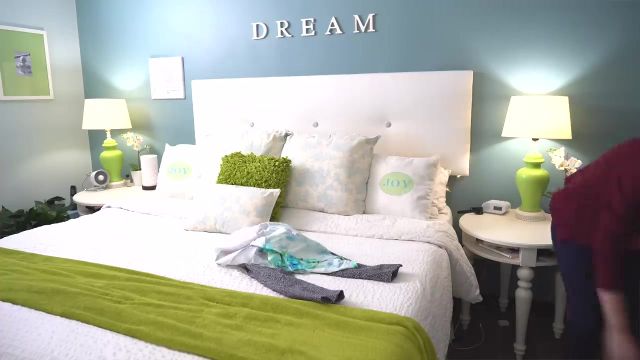 I owned it. Put it in a bag to toss or donate immediately. You are going to see amazing success when you declutter. There should never be a space in your home that you're organizing where something doesn't leave. Decluttering is key. So move from space to space one drawer. 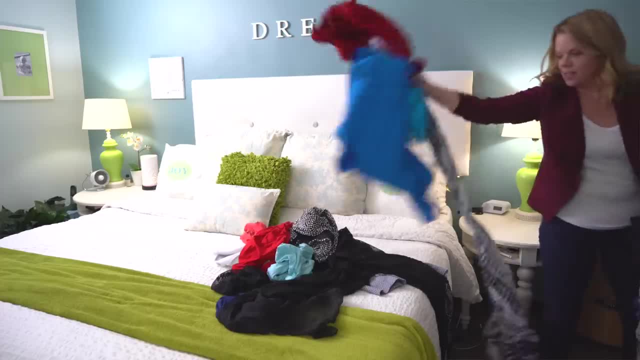 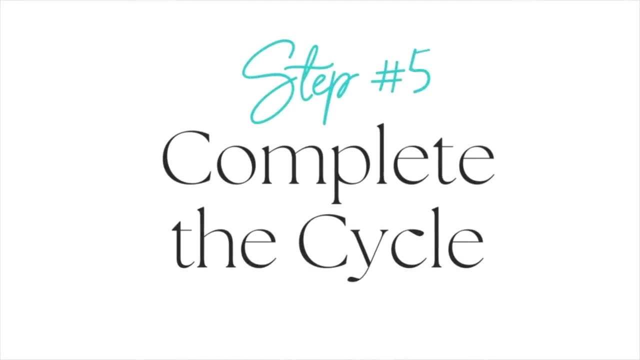 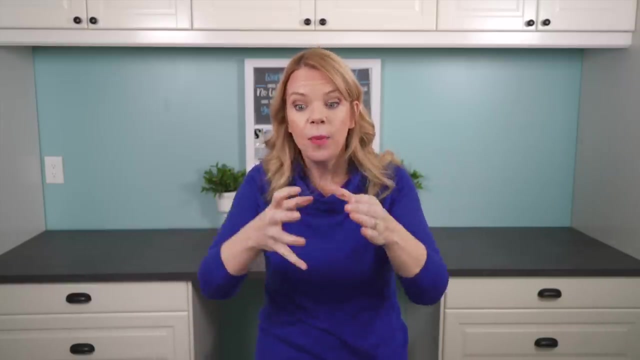 one project. whatever you have scheduled that day, organize one at a time and make sure you're decluttering along the way. Complete the cycle, And what I mean by this is: don't stop until you've tidied up any mess from organizing that. That's why we start with really small projects, Because what I used to do when 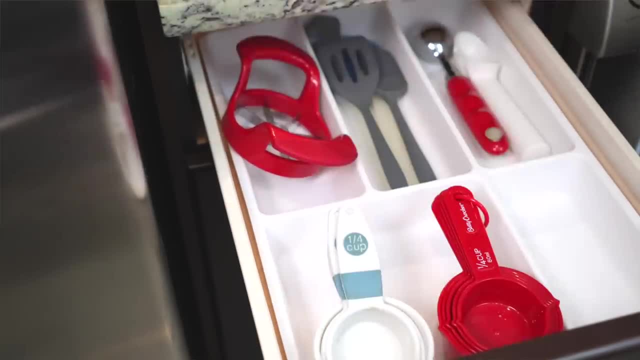 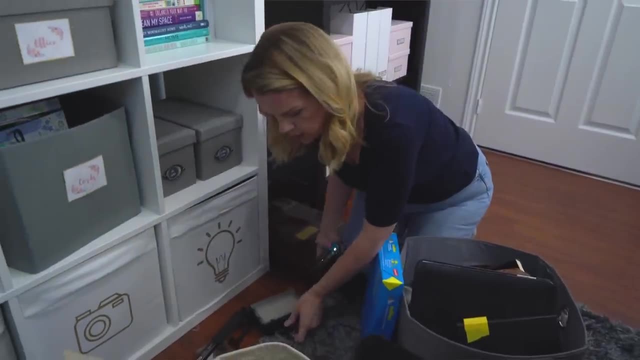 organizing was. I would start organizing a drawer and then there would be a ton of stuff that didn't belong in that drawer, but I didn't know where else to put it, So I would put it in a bag or a box and leave it to the side, And then I would have a ton of random clutter everywhere that I 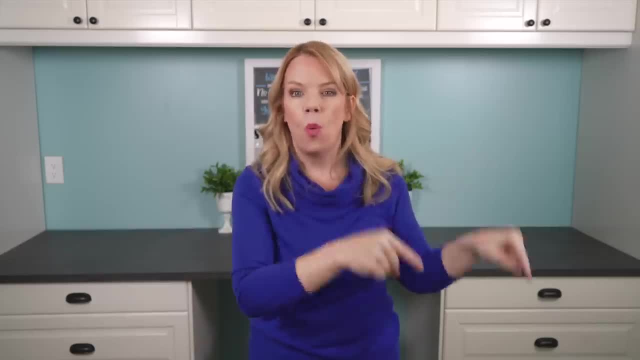 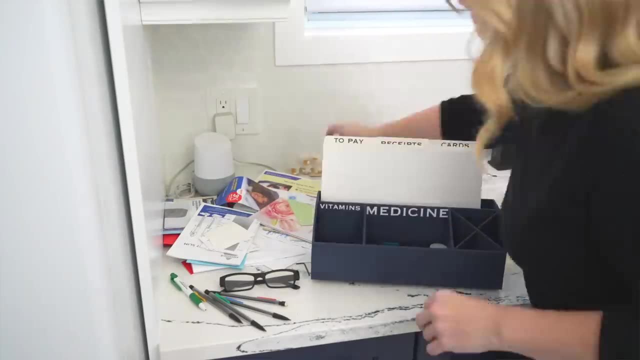 was going to put in. Completing the cycle means actually putting that stuff away. And if it doesn't have a home, you think where would I look for this first? And you put it there And we don't organize the space where we're putting it. That's not what this is about. It's about getting things. 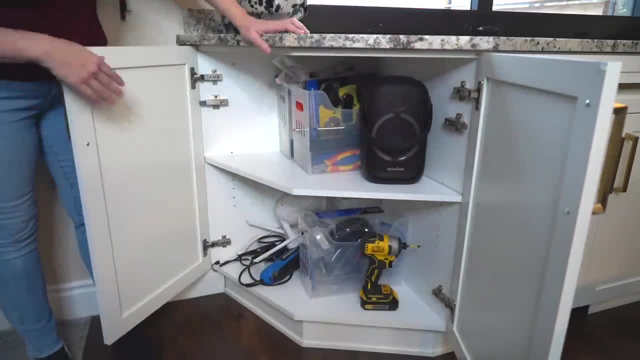 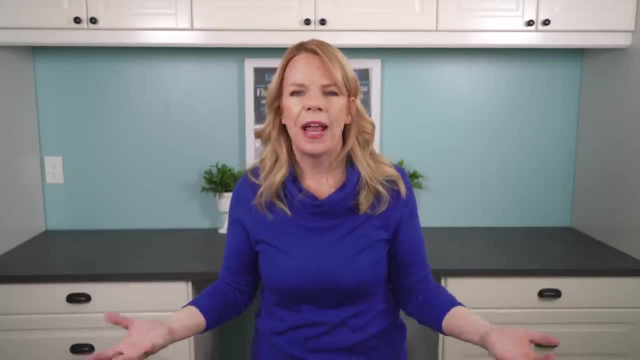 into a good enough home And if there are things that you're like, I honestly have no idea where I would look for this. I don't even know that I owned it. It's super random. It's like a little broken piece of plastic and you don't know what it's for. Get rid of it, It's not going to work. You're not going to get a new one, You're going to get a new one. So if you're going to get a new one, you're going to have to find a new one, And if you're going to get a new one, you're going to have to find a new one. 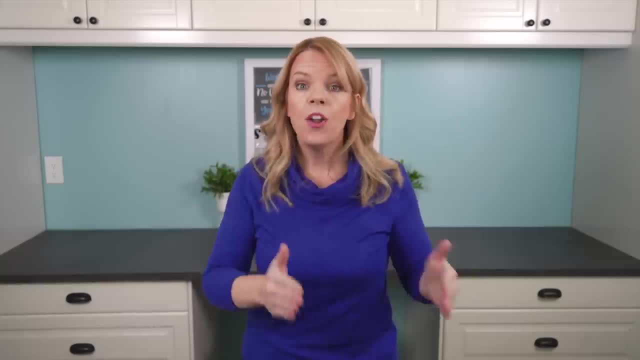 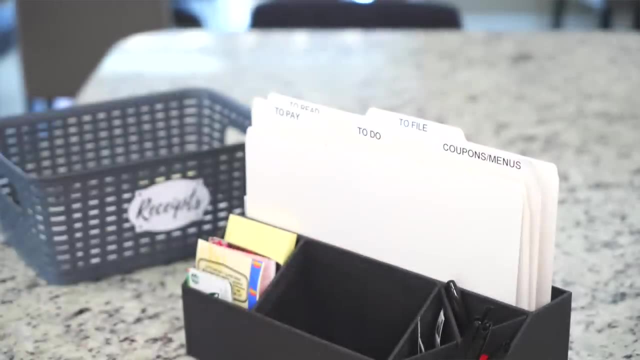 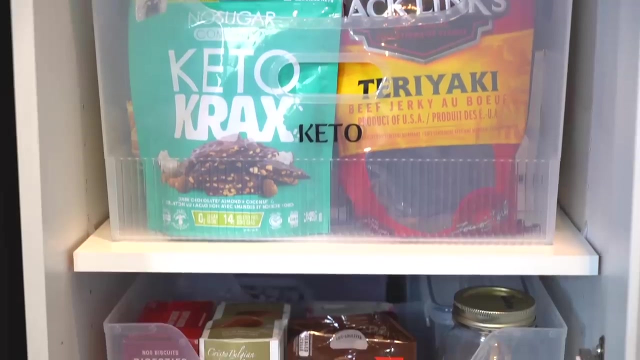 Get rid of it. Stop the stuff shuffling. You are not done until you're done. Finish each project, Do it. You will be, even if you're just putting things back into the drawer. we're not creating more mess for ourselves because we want to see progress. 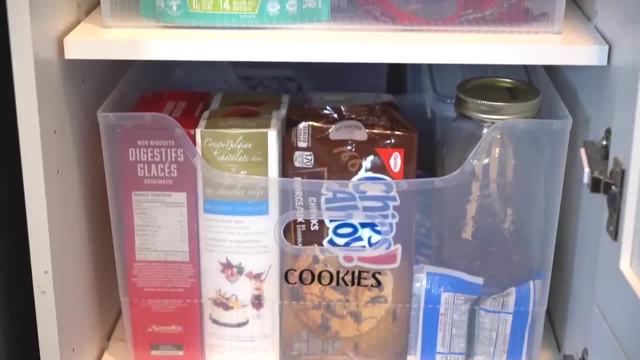 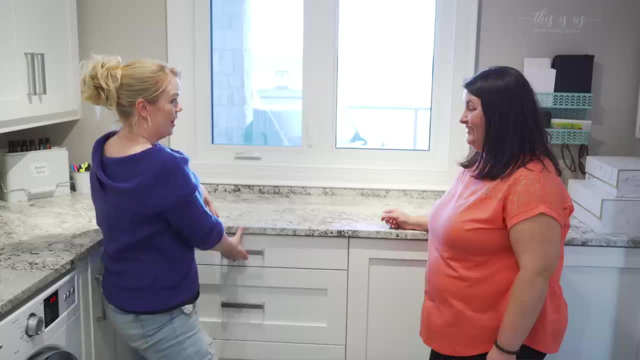 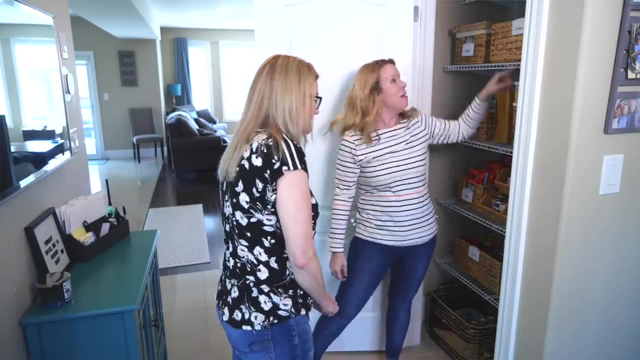 and nothing but progress. Completing the cycle is critical to having success when organizing your home. I've helped hundreds of clients organize their home, And the thing I find really fascinating is the people who struggle the most to get organized are almost always perfectionists. 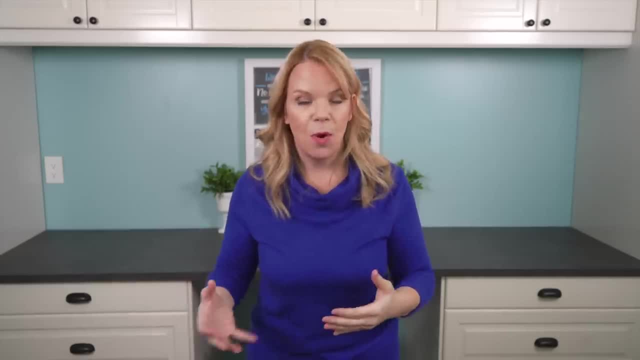 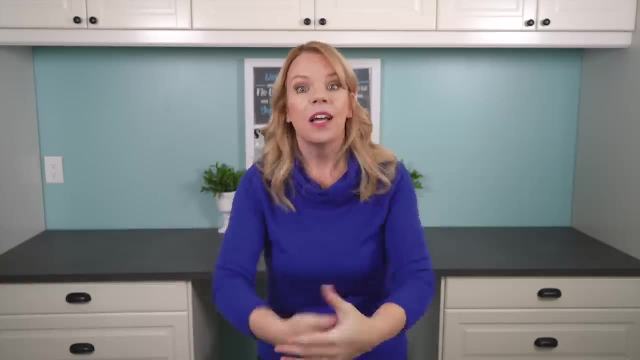 And they're really looking for the perfect solution. They want to buy exactly the right organizing tools, or they want to know exactly what it's going to look like when they're done. So they're reluctant to get started. But I'm here to tell you that it's that thought process that's. 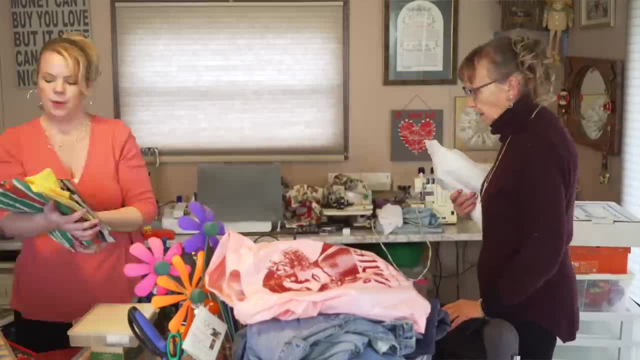 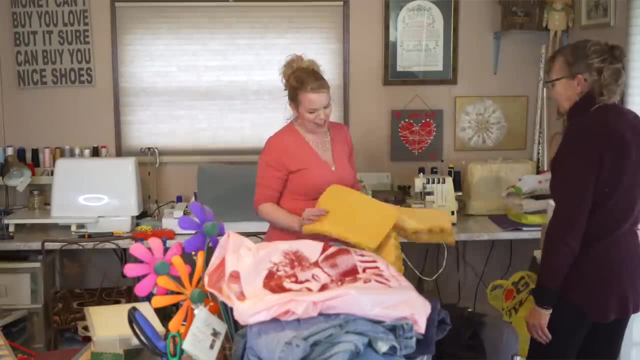 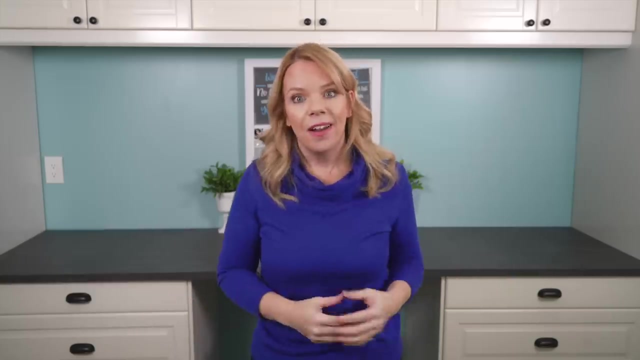 causing you to have a cluttered, messy home, And the way to overcome this is to embrace. good enough, Make a plan, Schedule time, Get started. It isn't about perfection. It isn't about making it Pinterest worthy. You look like some gorgeous Instagram thing. Getting organized is about having a 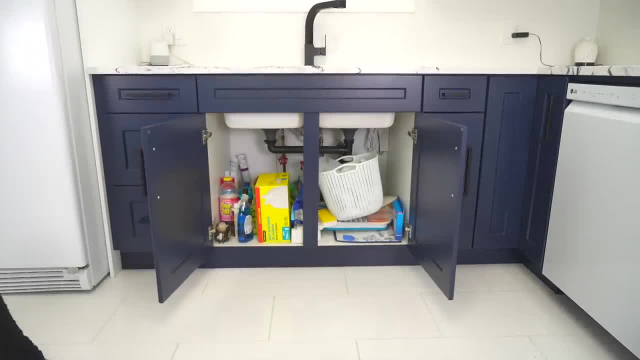 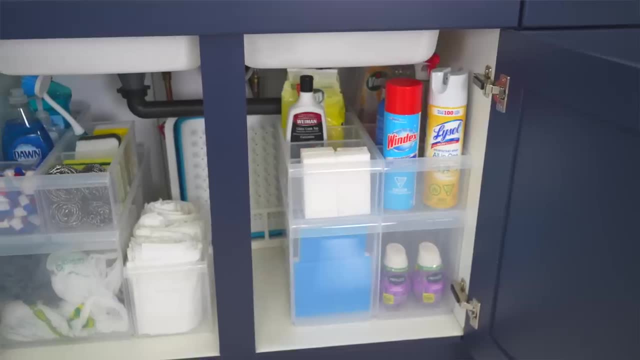 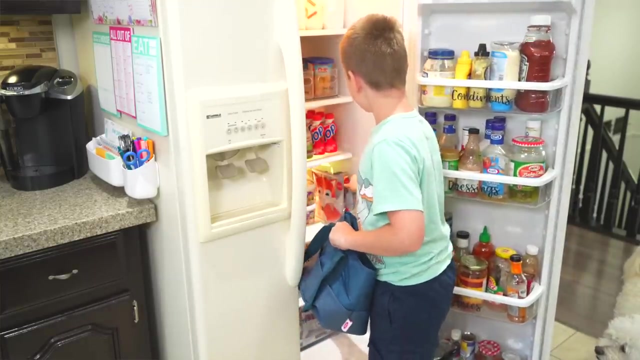 functional home that stays tidy, so you never lose anything. You know where everything is, You can find it in seconds And, even better, you and your entire family can put it away without even realizing that you're picking up after yourself. That is what organization is all about. 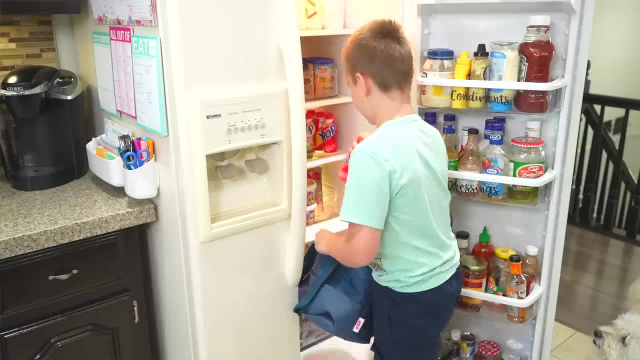 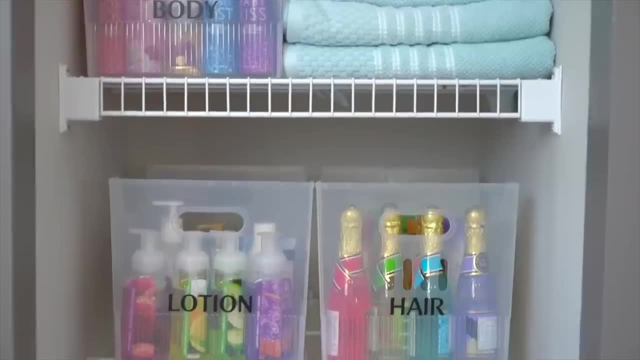 Once you've gone through and done your entire home, then we can go back and level up. Then we can buy beautiful containers and make it look the way that you're dreaming it looks. But that is the final step. That's like the cherry on top of home organization. It begins with a plan. 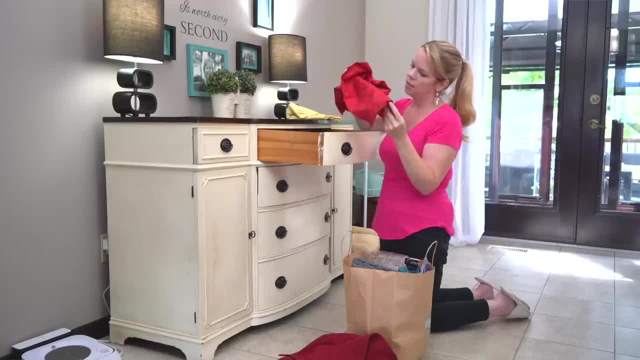 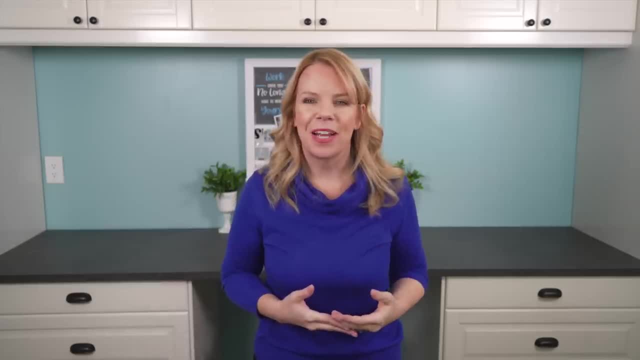 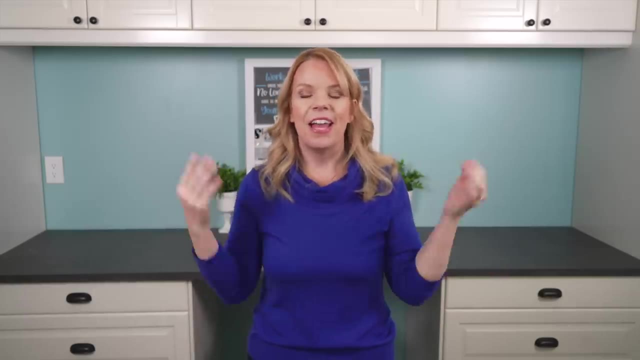 It begins with a meeting with yourself And it begins with letting a ton of stuff go. I hope you're feeling inspired to try again when it comes to home organization And if you do nothing else after watching this video, I hope you grab a piece of paper and a pen and you just 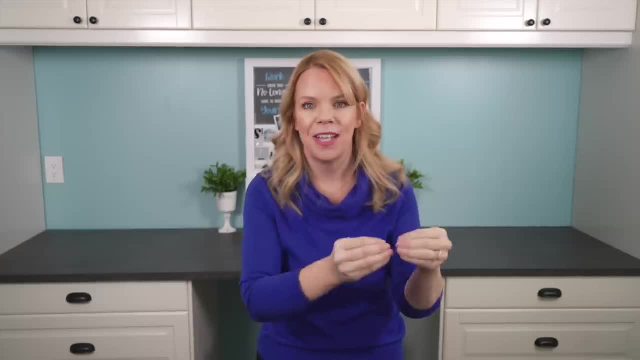 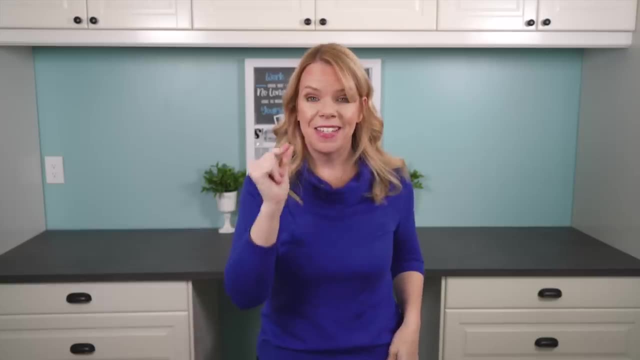 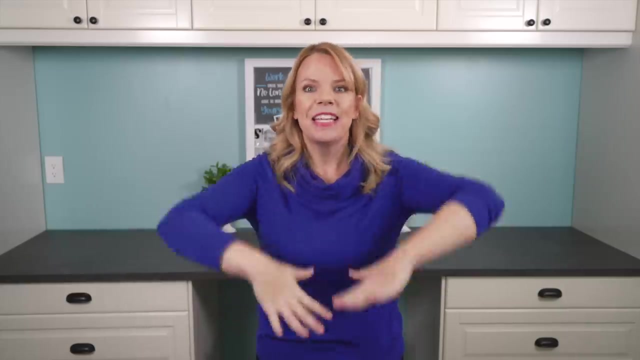 brain dump. Write down all the little projects that you want to do. Break them down into bite size, small steps, and then just pick one and schedule yourself to do it this weekend. Embrace that. good enough, you guys. You deserve this. And the best way to tackle a huge thing. 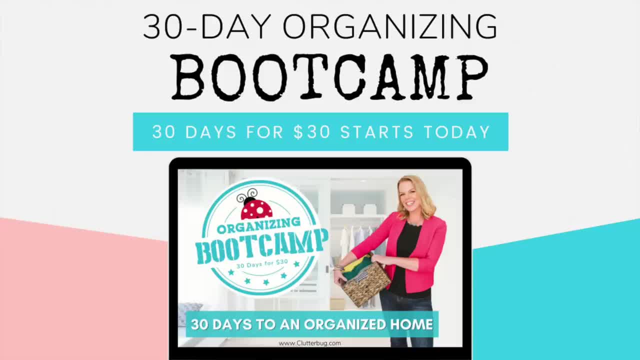 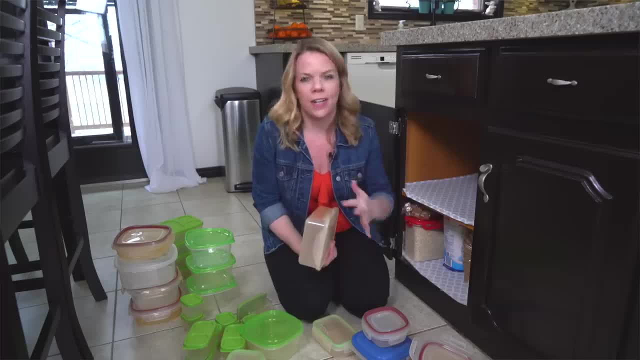 is one small step at a time. If you're looking for extra support and help, don't forget that I have a 30 day bootcamp that you can sign up. It's just a dollar a day, just $30 to transform every little tiny area of your home. I'm going to put the link in the 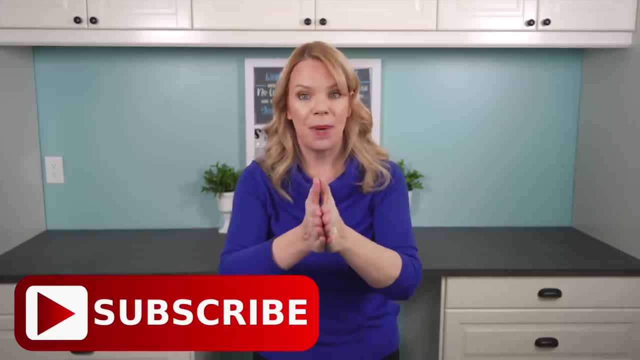 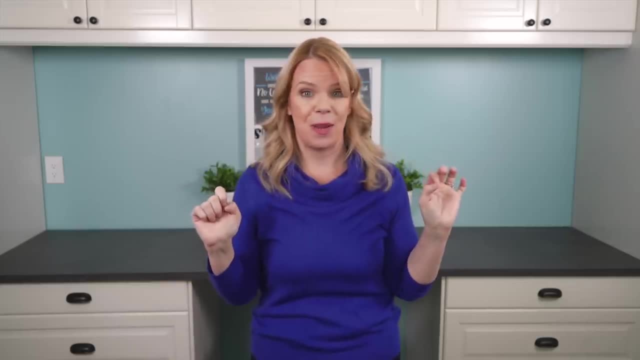 description below and make sure that you hit that subscribe button and come back, because, January, I have the amazing, incredible organizing transformations for you. I can't wait to show you. These are awesome And I will see you then. Hey guys, thanks so much for those of you who have. 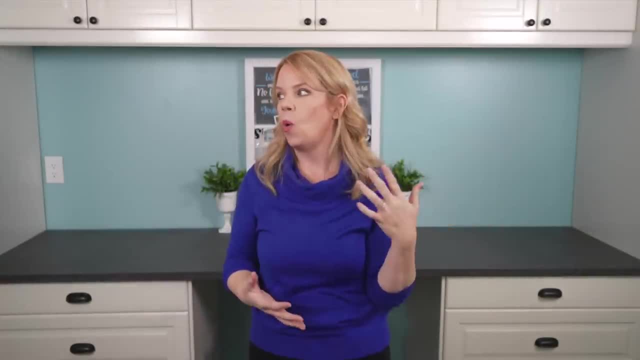 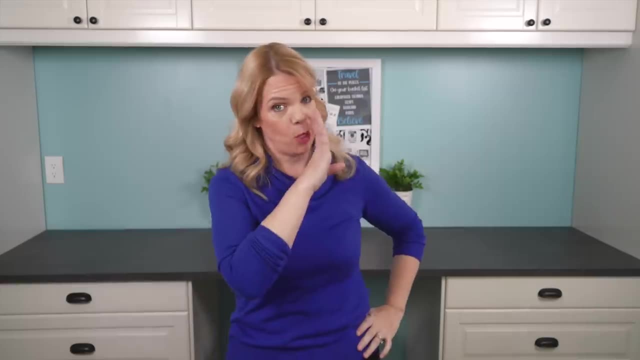 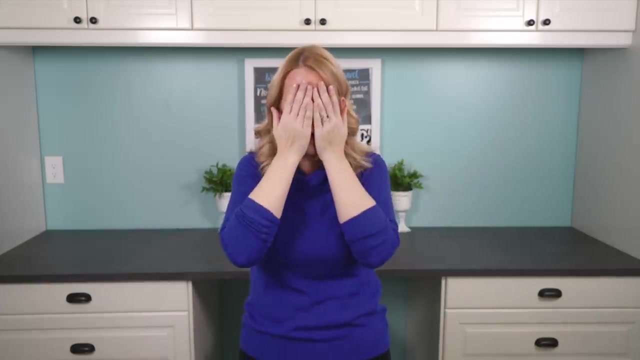 stayed to the end. If you've watched my channel for a while, you know that I'm a horrible driver, like the worst driver ever. I hit curbs. I've had to have multiple rim jobs because my rims are so bent on my car And I've hit carts. I've hit walls. I've hit buildings- Never another car, though. 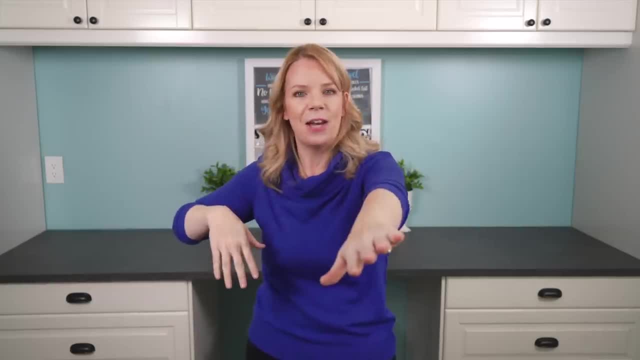 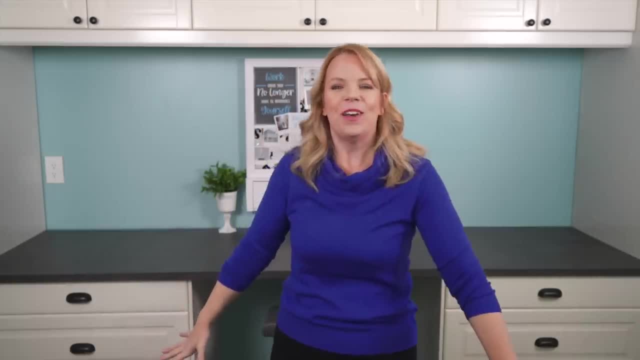 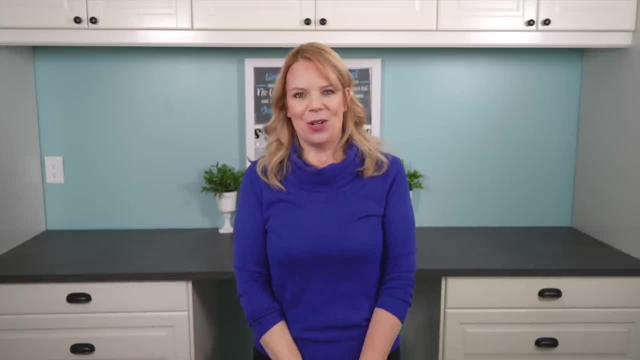 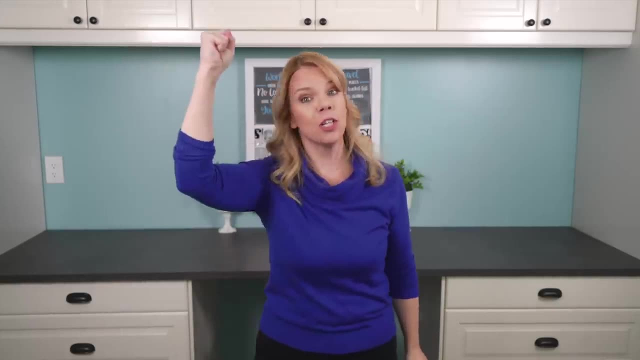 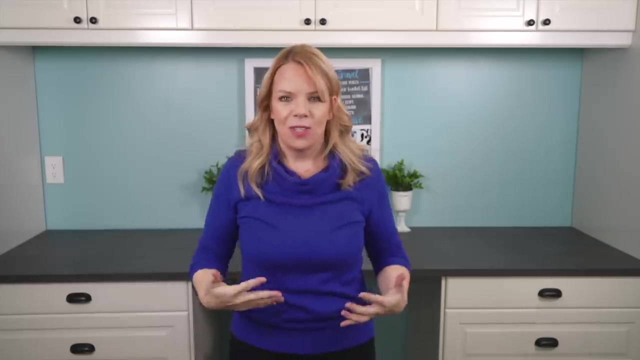 got it on the third and now it's teaching her to drive time. I have so much anxiety driving myself. Now I'm just holding onto the bar, gripping the thing and I find I'm like, oh, slow, go down, go. oh, I'm doing this the whole time So I don't know. 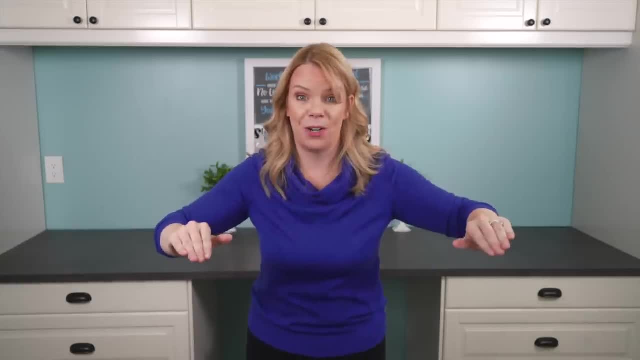 if you have taught a child to drive, Please give me your advice, because I don't want to pass my anxiety off to my phenomenal godproduct who taught me to drive? And also I don't want to pass my own солн까 FABIEN'S. I'm like we're going to have some fun too. And then, when I get older, I'm like: 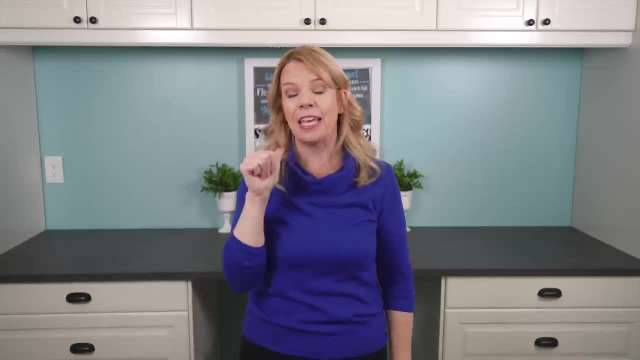 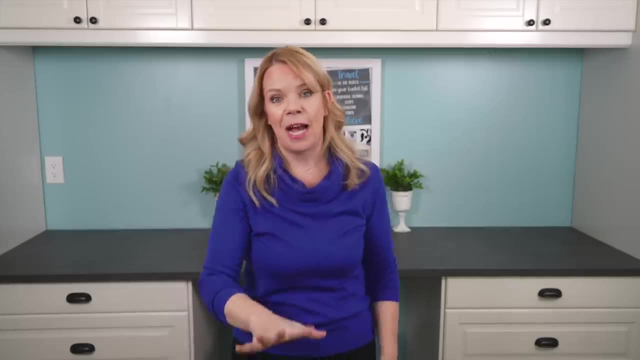 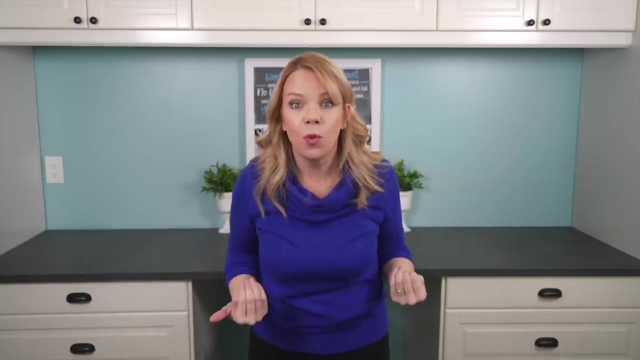 onto her but for some reason, when she hits the gas I get whiplash like you've never known, and when she breaks, I swear my face is going through the windshield every time. light foot Izzy, light foot Izzy. you can do it, and the cars are coming and I'm like and I forget the rules of the road. 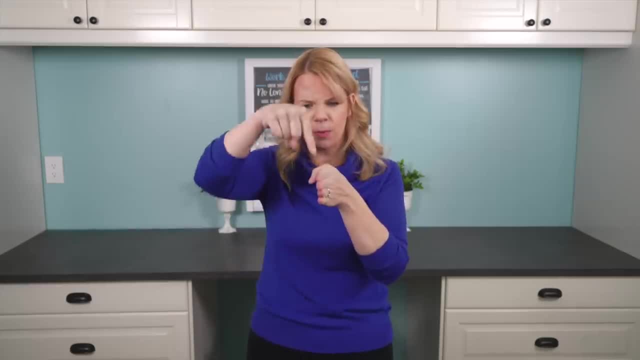 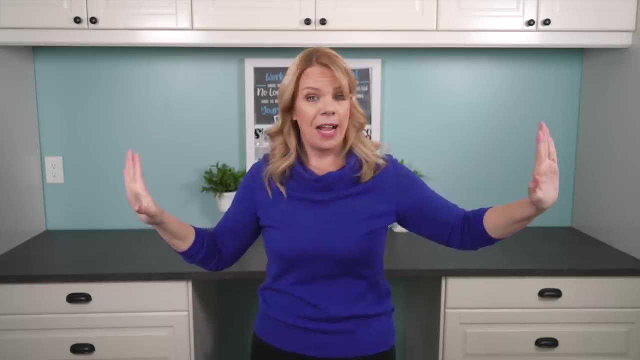 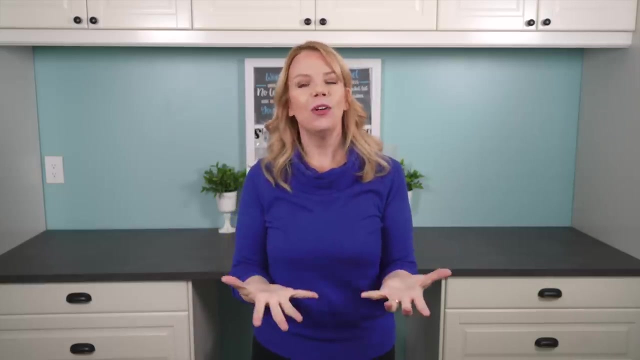 too like: can you go? and if you stop, I know it's the person and then the person on the right, but what if you both stop at the same time here? who gets to go first? it's a nightmare. okay, teaching a kid to drive has been the most stressful thing that I've done in a very long time, so I welcome. 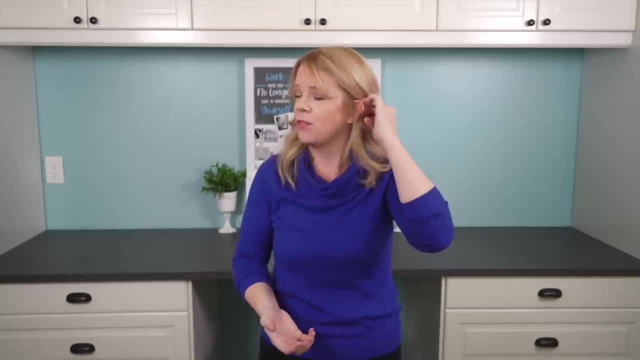 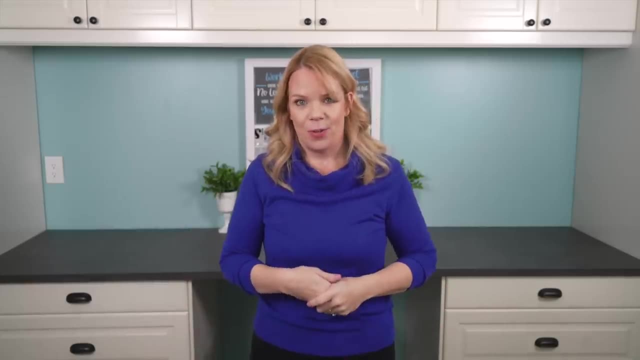 your advice. if you've done this, I think I might just pay for driver's ed. I think I might just pay someone else to teach her, so we both don't have a brain aneurysm. thank you guys, so much for watching and I'll see you next time.